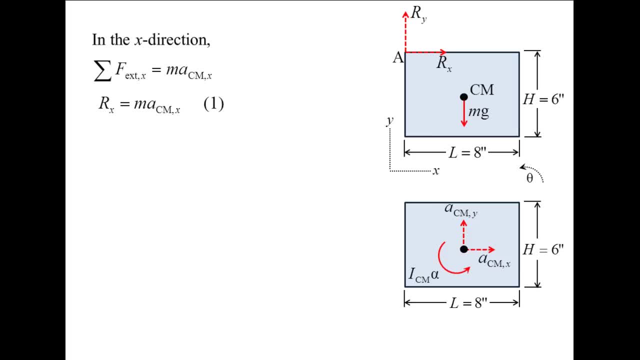 This is equation number one For the y direction. Ry is pointed in the positive y direction and the weight is pointed in the negative y direction. This is equation number two For the moment equation, the moment of inertia about the center of mass Icm. 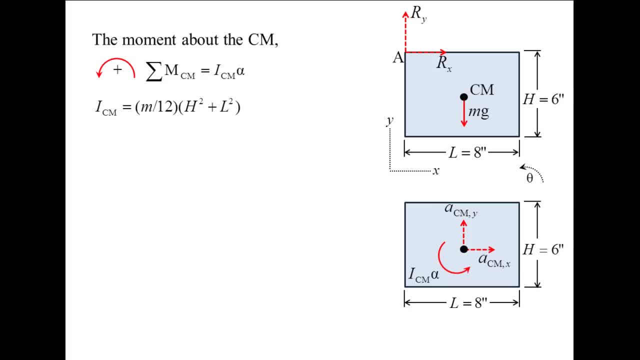 is the mass of the plate divided by 12, times the quantity h squared plus l squared. Next we determine the moments of the external forces about the center of mass. Rx produces a negative moment and has a moment arm of 1 half h. 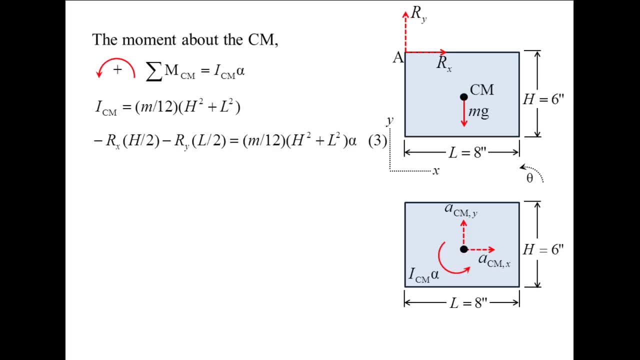 Ry produces a negative moment and has a moment arm of 1 half l. The weight produces no moment because its moment arm is zero. We now have equation number three. We have used the three equations of motion but have five unknowns. 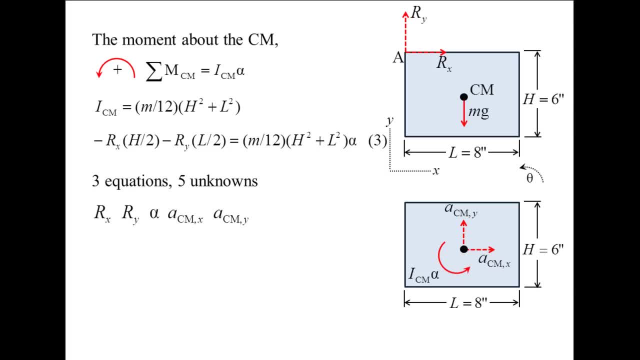 Rx, Ry, alpha and the two components of the acceleration of the center of mass. We can obtain two additional equations by examining the relative motion between point A and the center of mass. The acceleration of the center of mass is equal to the acceleration of point A. 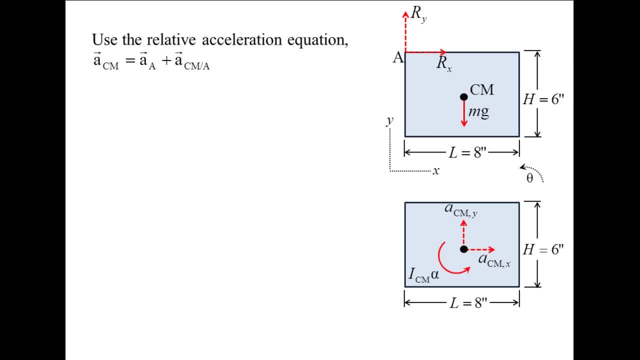 plus the acceleration of the center of mass relative to point A. The relative term is decomposed into tangential and normal components. The tangential component is alpha, cross, rCma, the position vector pointing to the center of mass from point A. The normal component is the angular velocity of the plate, omega. 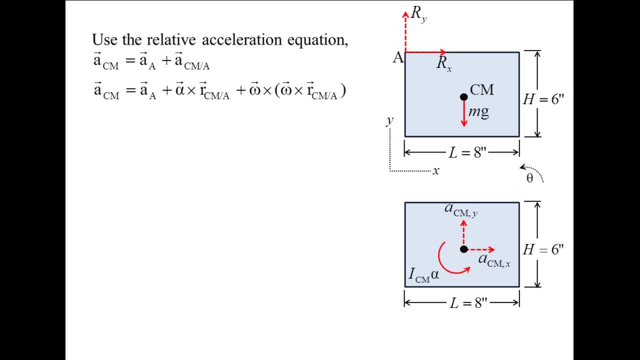 cross the quantity, omega cross rCma, The acceleration of point A is zero since that point is fixed. The angular velocity also is zero at that instant, since the plate starts from rest. The angular acceleration vector has the magnitude of alpha and points in the z direction. 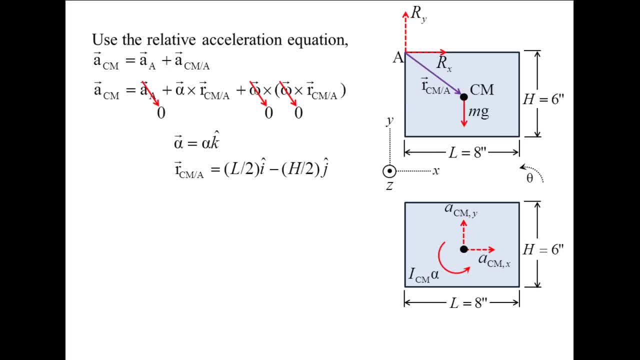 rCma starts at point A and terminates at the center of mass. The center of mass is located 1 half l toward the right and 1 half h downward from point A. Take the cross product on the right hand side of the equation.